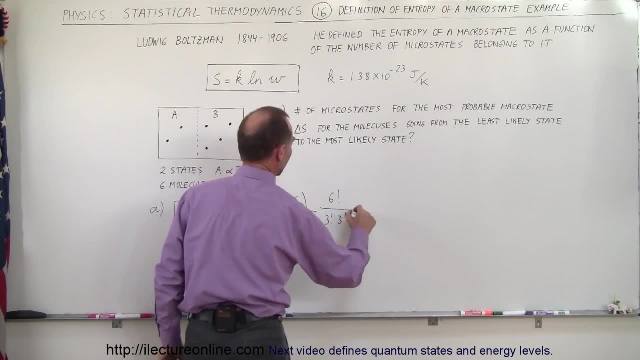 factorial divided by three factorial times three factorial. So this is going to be equal to six times five times four. divided by So three factorial will take care of the three, two, one, and then we still have the other three factorial like that, So six and six. 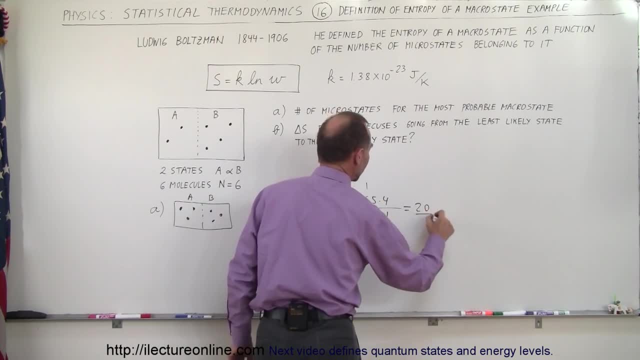 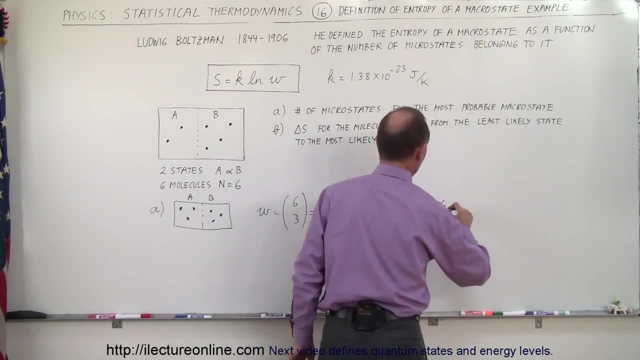 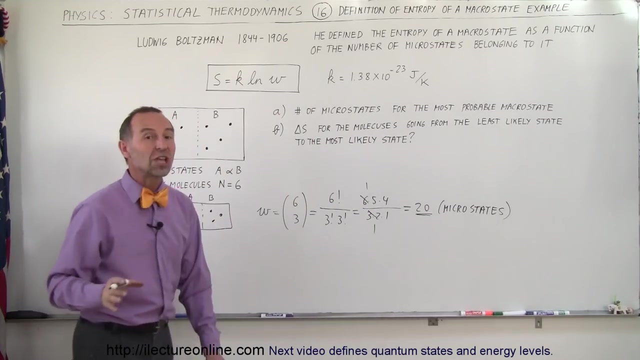 cancels out. This is one and one. So this gives us 20, which means there are 20 microstates for the most probable microstate. So 20 microstates. Secondly, we have to calculate the change in entropy going from the least. 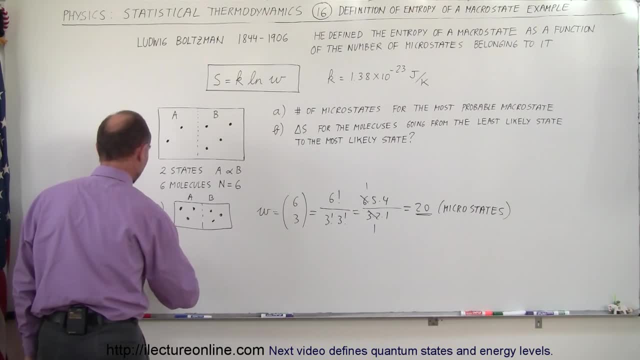 likely state to the most likely state. So for part B, the least likely state would be that all of the six molecules will reside in one of the two compartments. So it's either in the left compartment Or the right compartment, Doesn't matter. Two, four, I got one too many in there. So 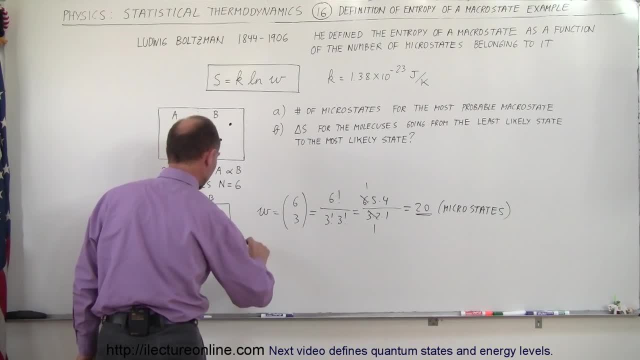 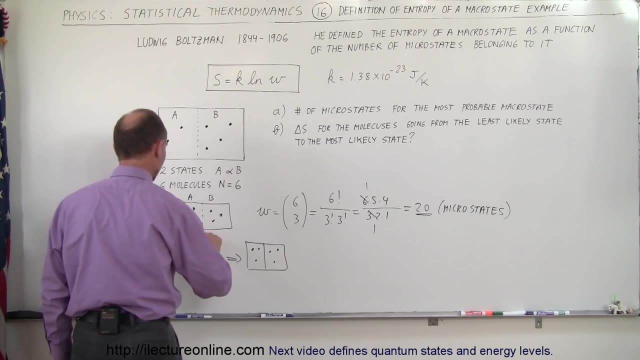 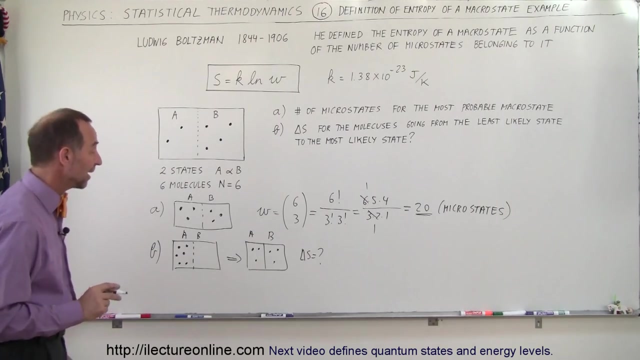 six in one, And then we go from this condition to this condition where you have the most probable state, where you have three in each. So this is A, this is B, This is A, this is B, And what is the change in entropy equal to? So what we want to do first is find out. 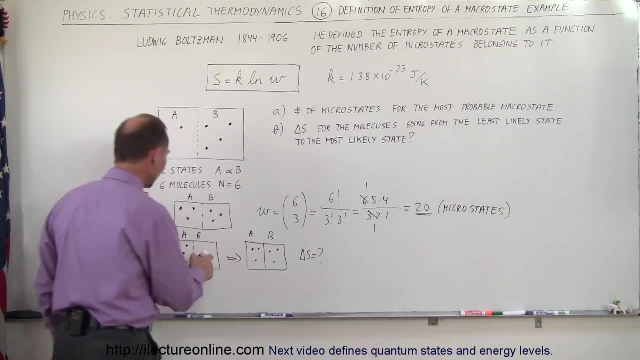 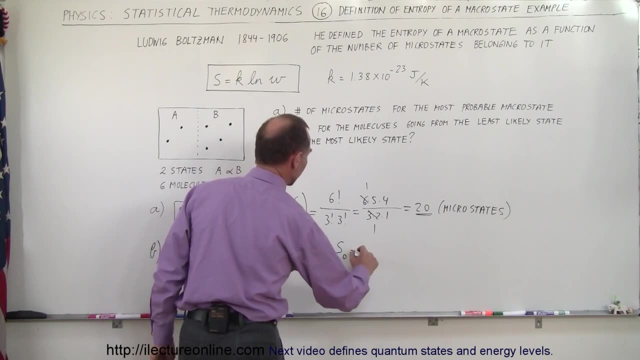 what the entropy state is of this. So in this case there will only be one microstate of this particular microstate macrostate. So we could say that S initial is equal to, according to the equation, the Boltzmann constant times, the natural log of the number of macrostates which, in this case, 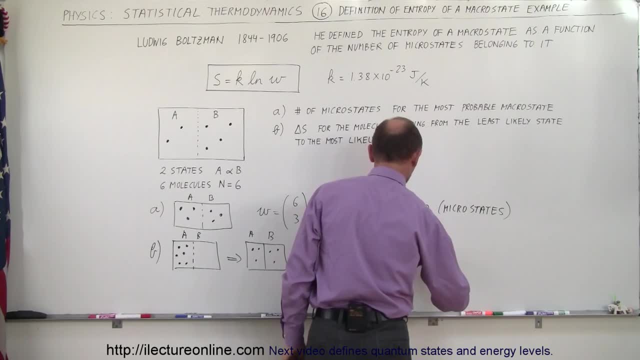 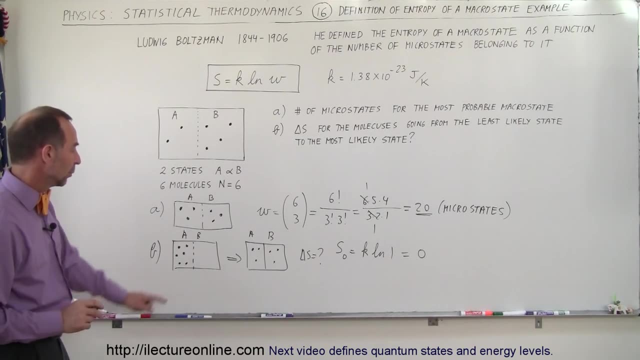 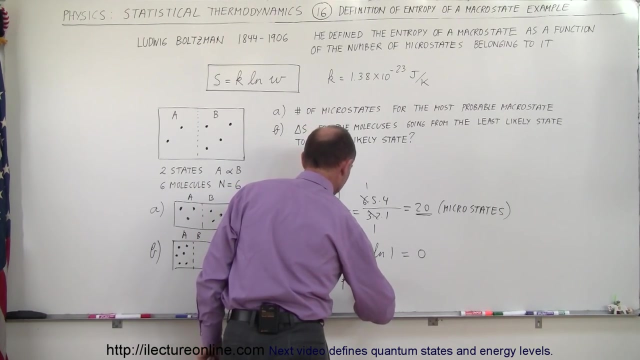 would be 1.. And so the natural log of 1 is 0,. so this would be 0. So the entropy would be 0. for the least likely state, which would be all 6 in one or the other compartment, The final entropy S final would be equal to K times the natural log of the number of. 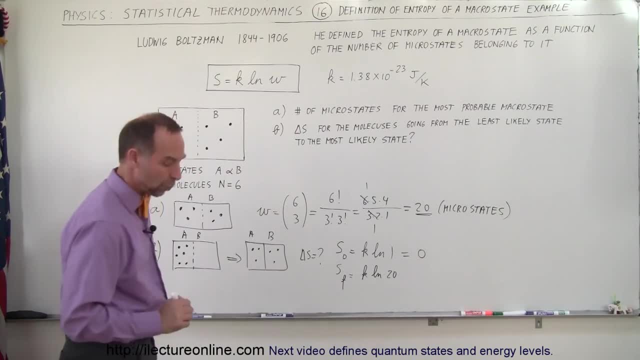 macrostates, which is 20.. So the natural log of 20, so we can say 20, take the natural log of that and that would be 2.96, so this would be equal to 2.96 K and of course the 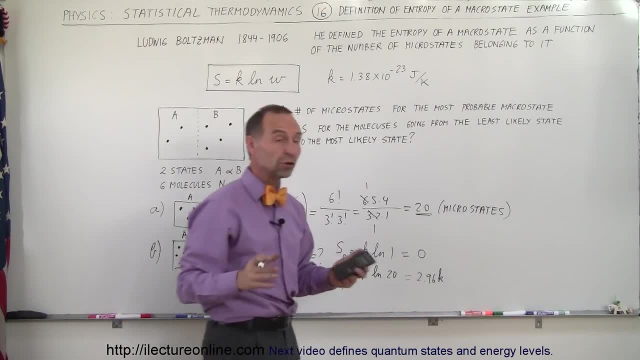 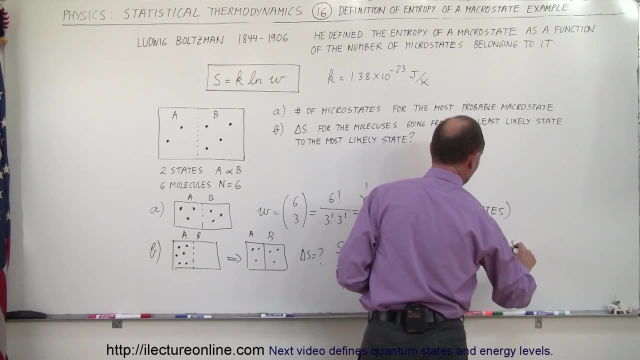 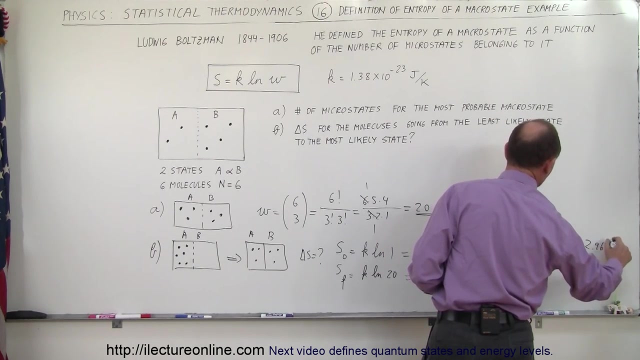 units would be K would be joules per Kelvin and those are the units for entropy. So the difference, the delta S, would be equal to S final minus S initial, which is equal to 2.96.. 2.96 K minus 0,, which is 2.96 K. or if you want to leave it like that, you could say: 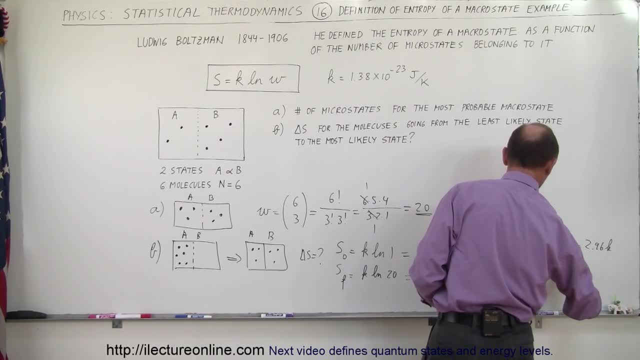 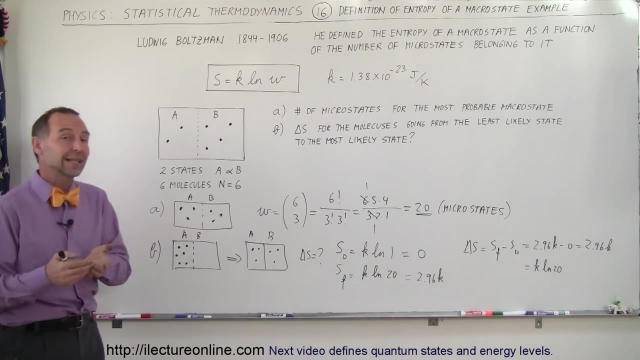 this is equal to K times the natural log of 20.. So either one would be the proper answer for that particular example. So that's how we do that. that's how we calculate the entropy of a simple example like that, and of course it would work for a more complicated example as well. But this is a nice way to 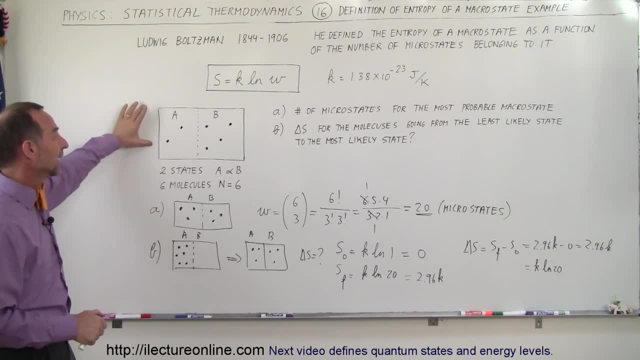 introduce you to how we can calculate the number of macrostates in a two-state system, calculate the entropy change when we go from one state to another, and that is how it's done. 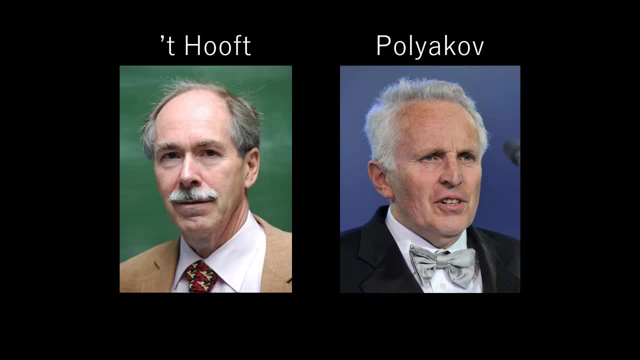 The symmetry between electric and magnetic fields in the source-free Maxwell's equations naturally suggests that electric charges might have magnetic counterparts known as magnetic monopoles. The prediction of grand unified theory gut monopoles arises from the work of T Hooft and Polyakov, who showed that certain spontaneously broken-gauge theories have non-singular classical solutions that lead to magnetic monopoles in the quantum theory. 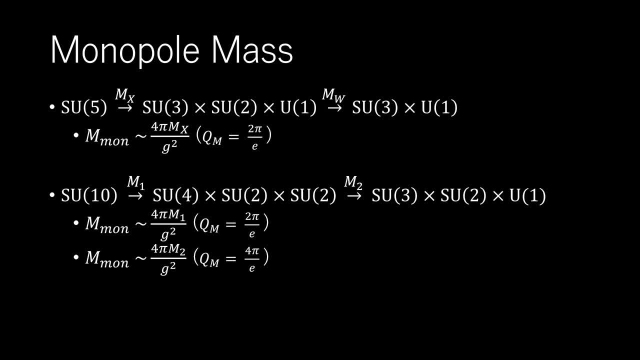 The monopole mass is determined by the mass scale of the symmetry breaking. that allows non-trivial topology. For example, an SU5 model with SU5 goes to SU3 cross, SU2 cross U1, and then goes to SU3 cross. U1 has a monopole with Qm equals 2π over E and mass m is approximately equal to 4πmx over G squared, where G is the SU5 gauge coupling. 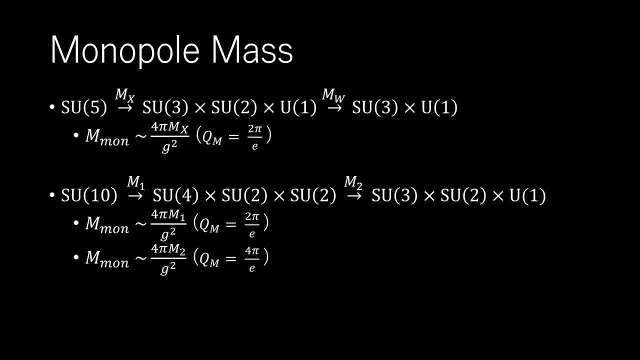 For a unification scale of 10 to the 16th GeV, these monopoles would have a mass approximately equal to 10 to the 17th to 18th GeV. In theories with several stages of symmetry breaking monopoles of different mass scales can arise. 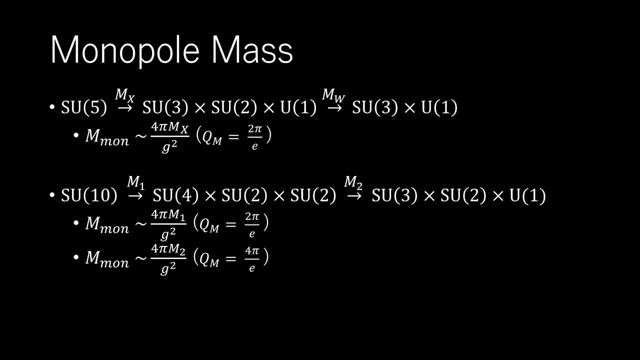 In an SO10 theory, with SO10 goes to SU4 cross, SU2 cross SU2, and then goes to SU3 cross, SU2 cross U1, there is monopole. with Qm equals 2π over E and mass m is approximately equal to 4πmx over G squared, where G is the SU5 gauge coupling. For a unification scale of 10 to the 16th GeV. these monopoles would have a mass approximately equal to 4πmx over G squared and a much lighter monopole with Qm equals 4π over E and mass m is approximately equal to 4πmx over G squared, where G is the SU5 gauge coupling.